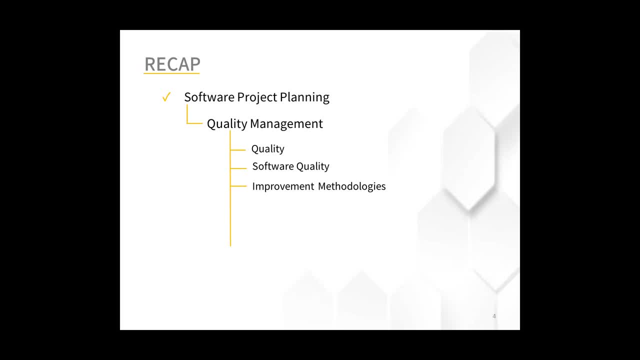 and then we deep dive into that. So from that we were able to talk about the three main factors driving quality management. We discussed different improvement methodologies that helps promote quality management. We also discussed that- how Toyota earns the title of king of total quality management. 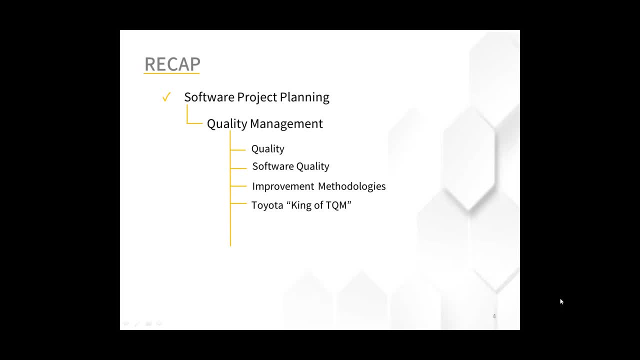 we also talked about one of the most important technique improvement technique. that is Kanban. how can man helps in software quality management? in last we started with three main activities of software quality management. that are number one, software quality assurance, number two, software quality planning and number three. 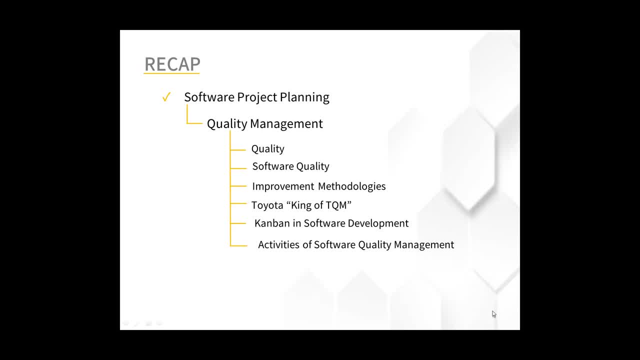 software quality control. due to time constraint, we can explore only the first activity of software quality management. that was software quality assurance, and we will talk about the rest of the activities. so we discussed in detail about software quality assurance, as software quality assurance is the activity of selection and definition of standards will distinguish between: 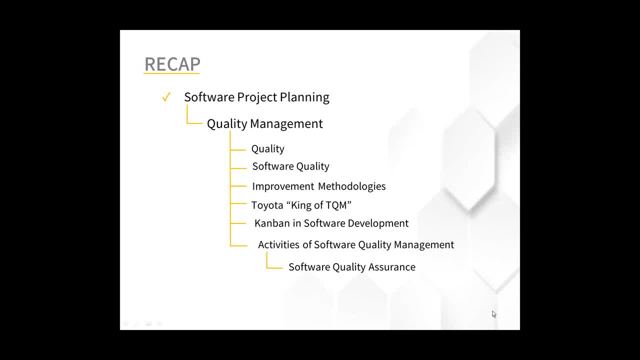 products and services. we will talk about the first activity, which is software quality management, and the second activity, which is software quality, product standards and process standards. While talking about quality assurance standards, we also discuss ISO 9000, an international set of standards that can be used in development. 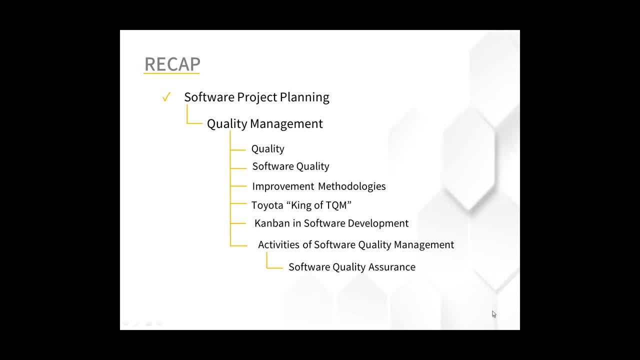 of quality management system in different industries. So let's start with our today's lecture. So in today's lecture, first we will complete our discussion on our remaining activities of software quality management, that are, software quality planning and software quality control. Then we will learn about different factors that influence software. 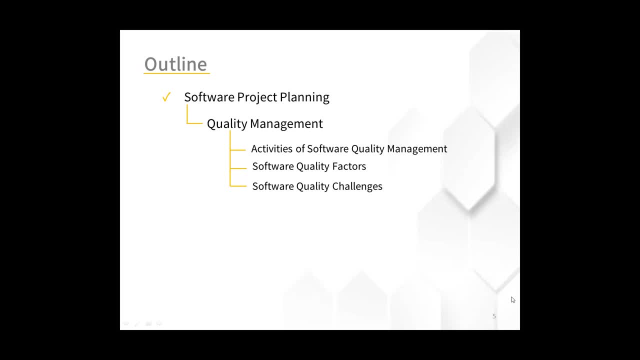 quality. After that, in this lecture, we will also highlight different challenges that software industry is facing. So let's start So, as we are done with software quality assurance, we will switch directly to our second activity of quality management, that is, software quality. 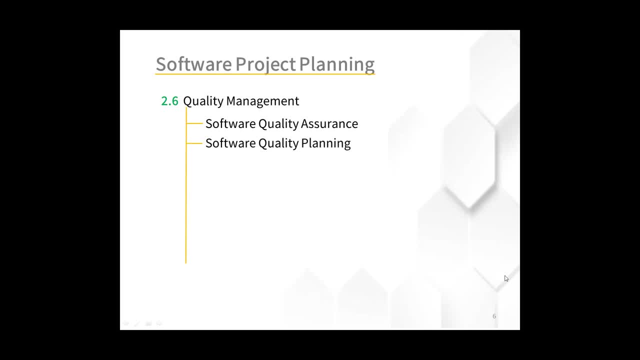 planning. so what is quality planning? quality planning, or software quality planning in simple words, is the process of developing quality plan, quality plan for our software project, system project. in software quality planning we basically identify all the requirements of our software project at the very beginning of our project. we also figure out how we can measure these requirements or how we will. 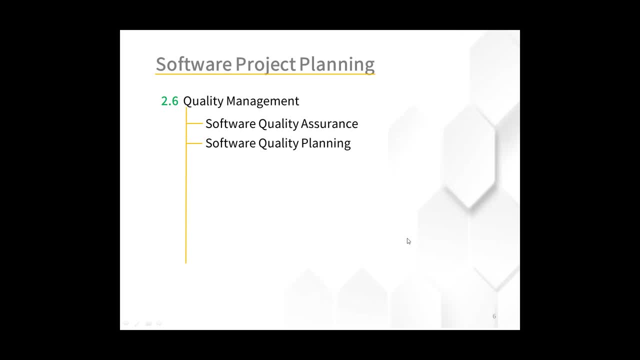 measure these requirements and we can prevent defects in our software project. we can divide our software quality planning into five main activities. number one is software. sorry, we have to mention all the objectives of our product. we have to mention all the characteristics, specification, cost, time, resources, scope and stuff like that. we have mentioned all these. 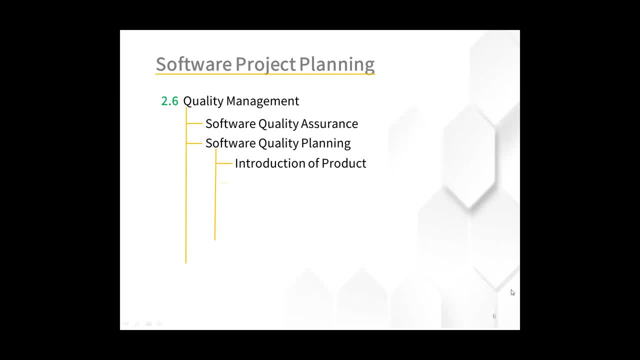 things in introduction of product. next step is product plans. product planning is a very difficult term to define because it's a very broad term. it encapsulates so many things. so, but briefly, we consider product planning involves all the internally focused decisions, steps and tasks that will be necessary to develop a successful product, like what features should. 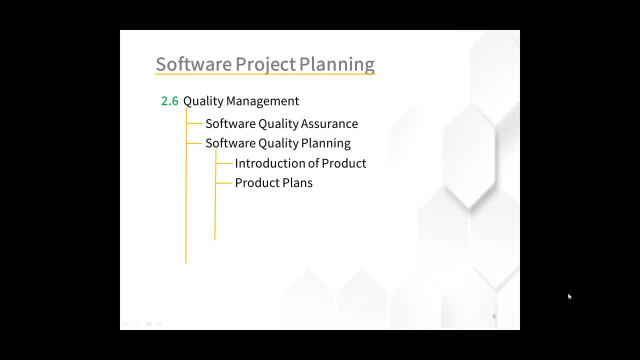 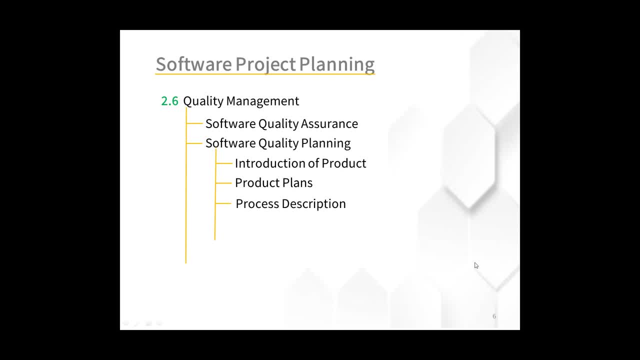 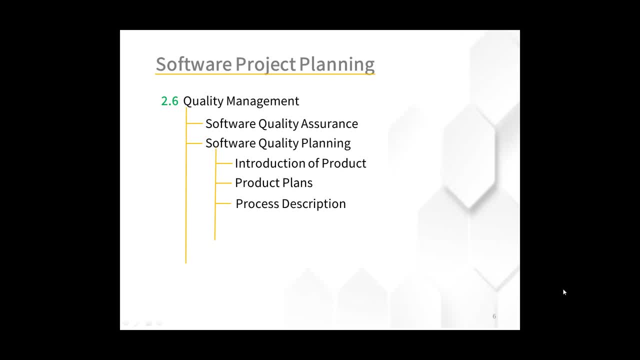 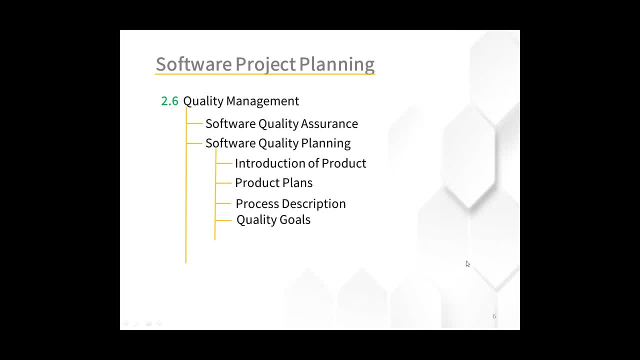 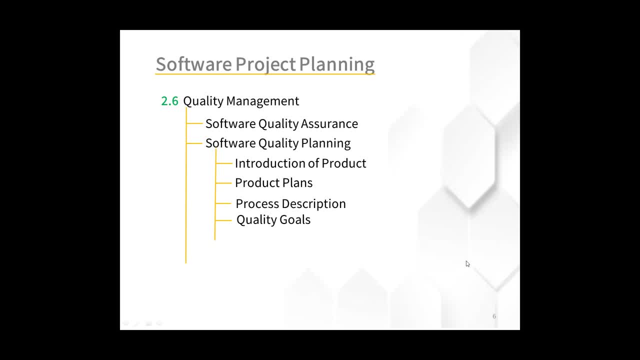 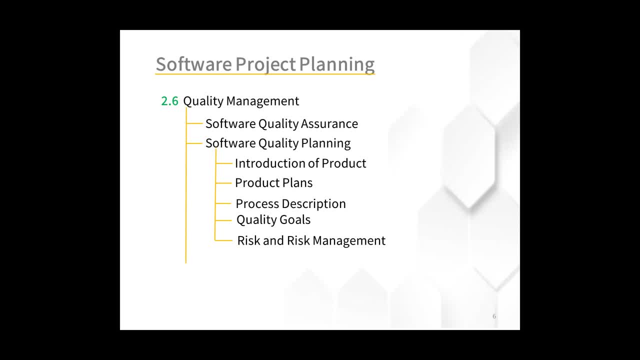 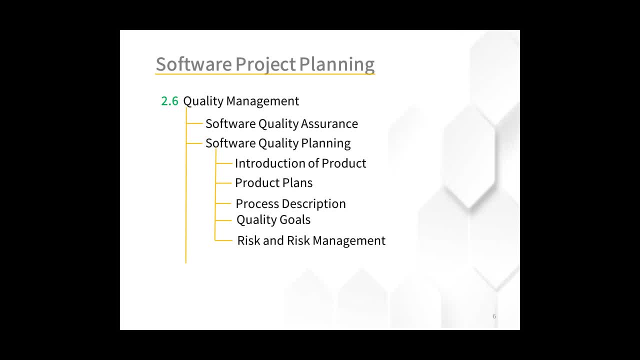 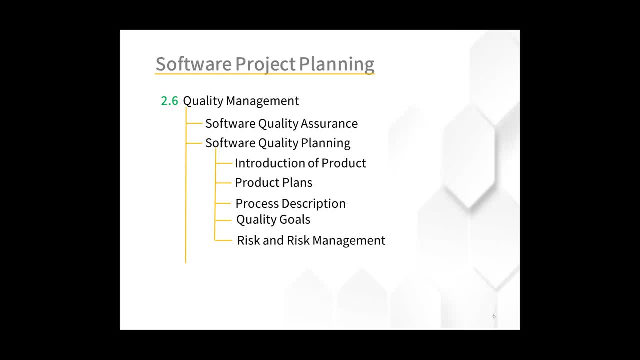 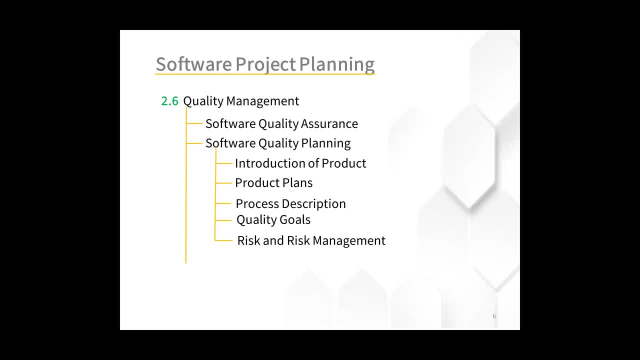 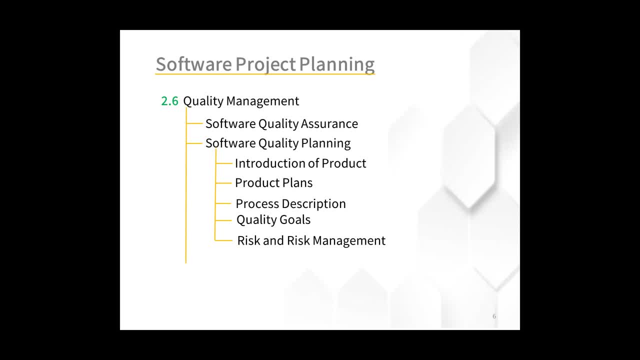 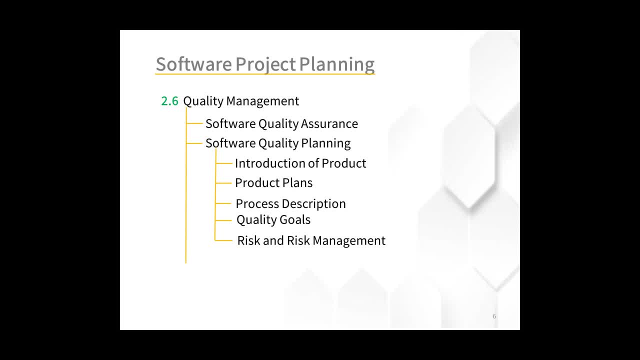 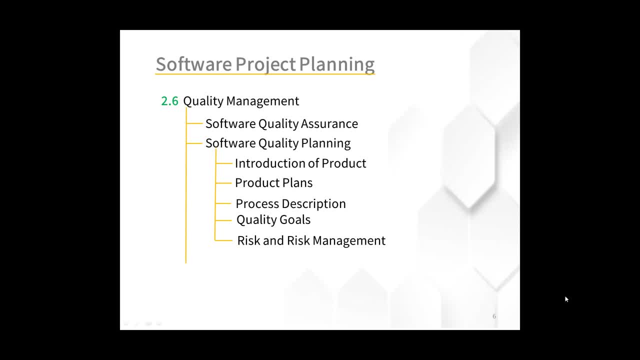 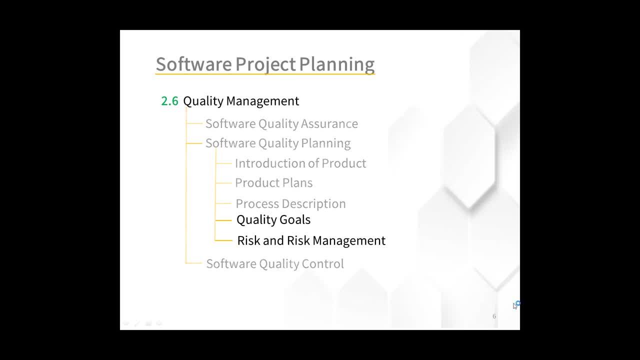 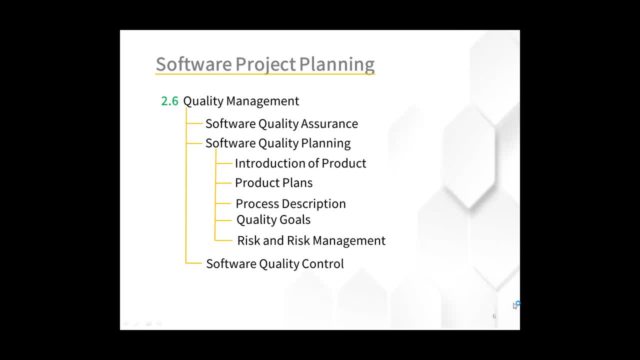 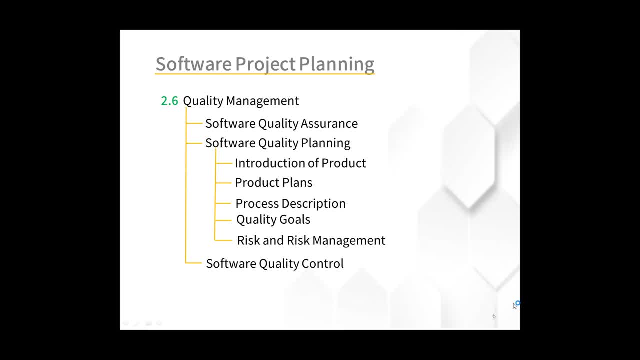 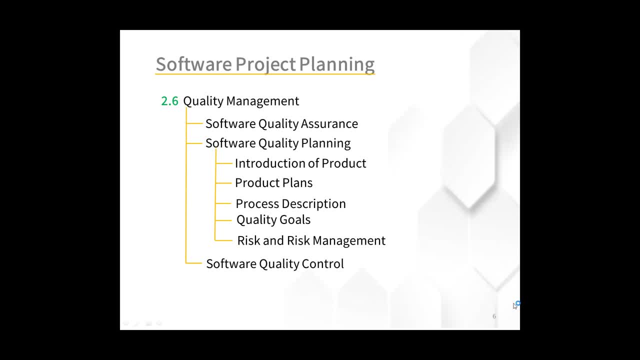 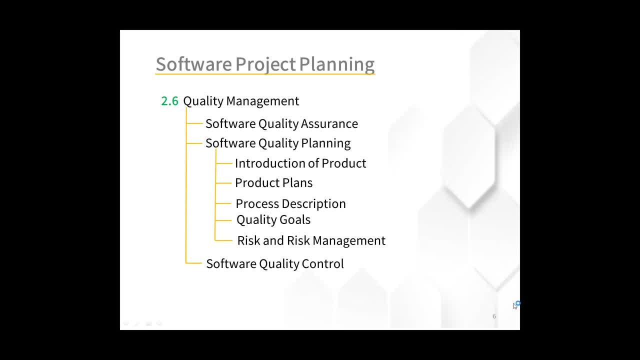 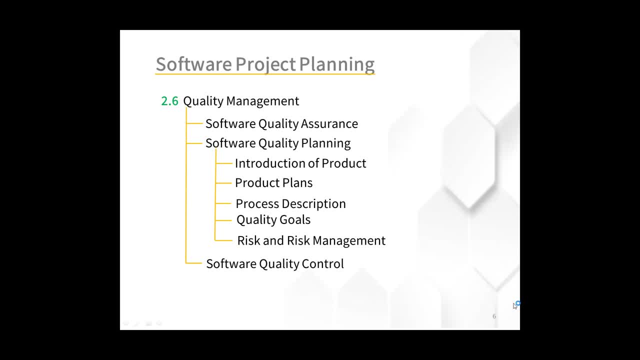 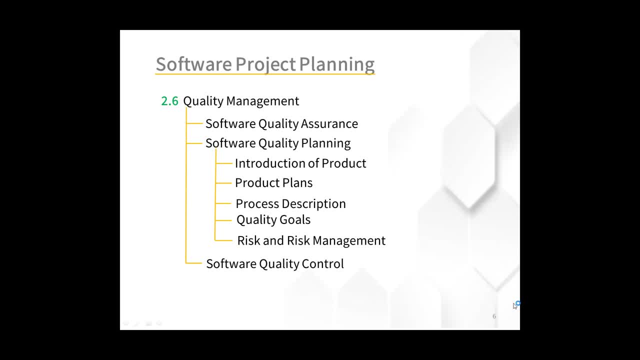 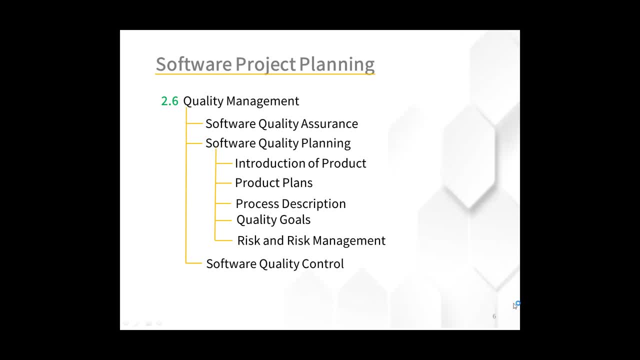 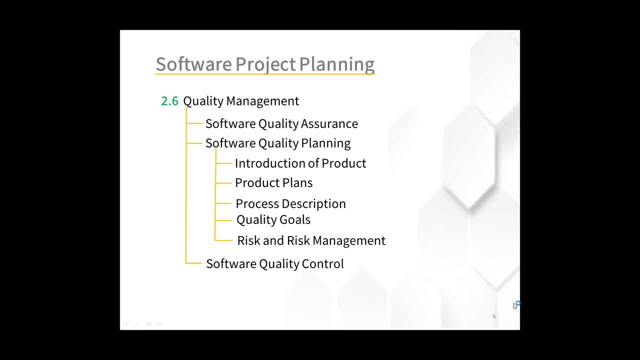 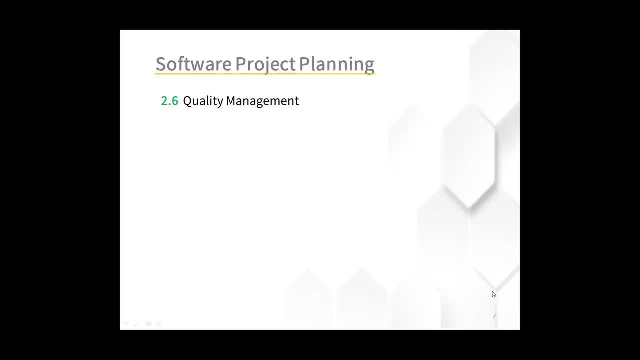 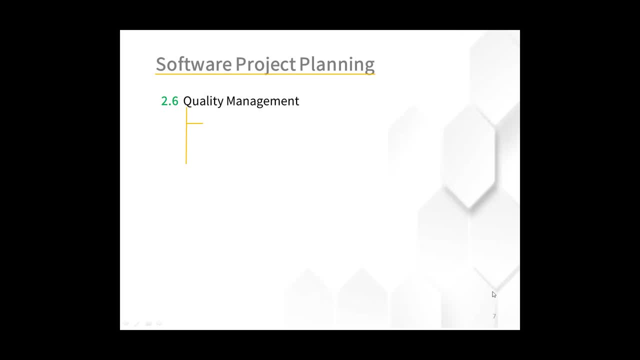 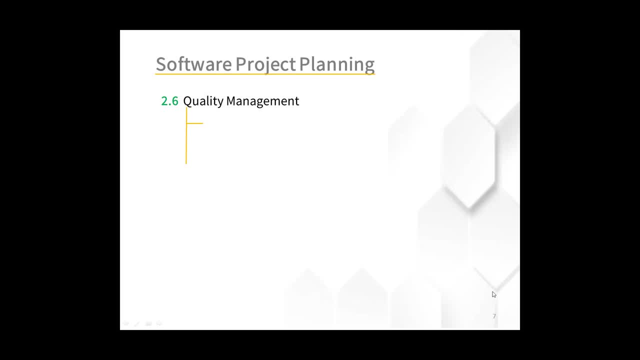 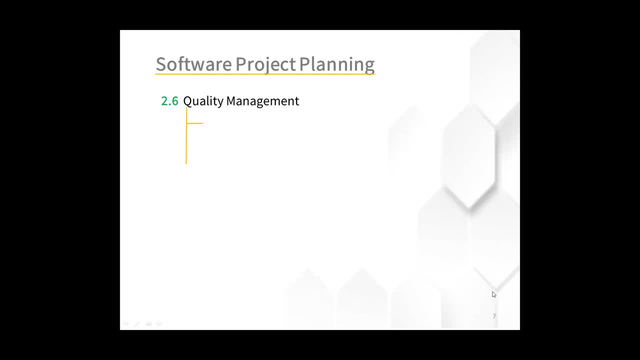 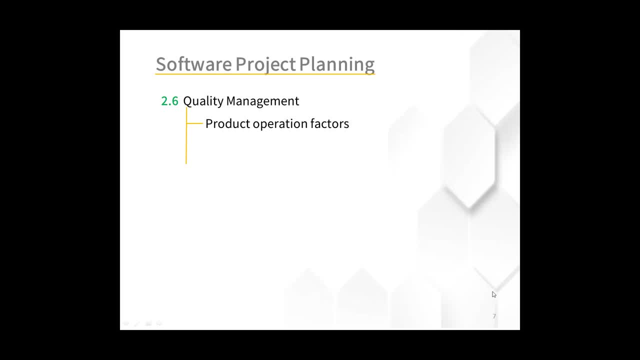 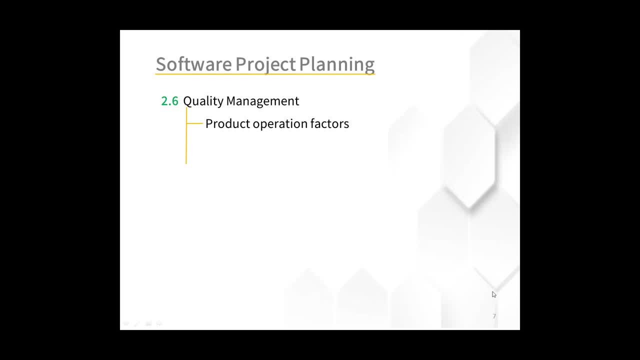 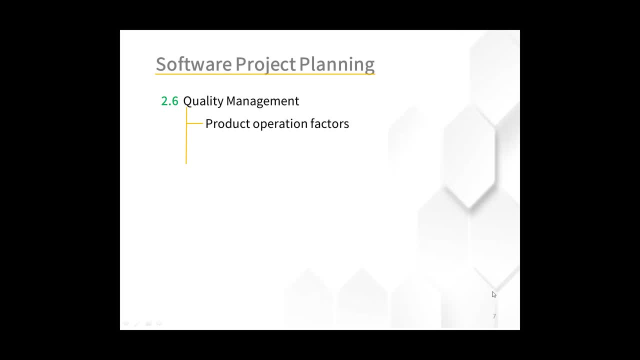 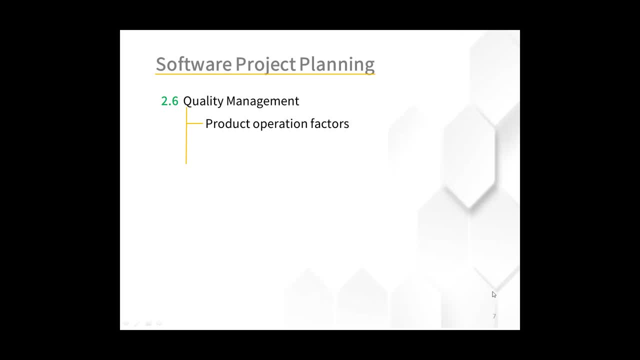 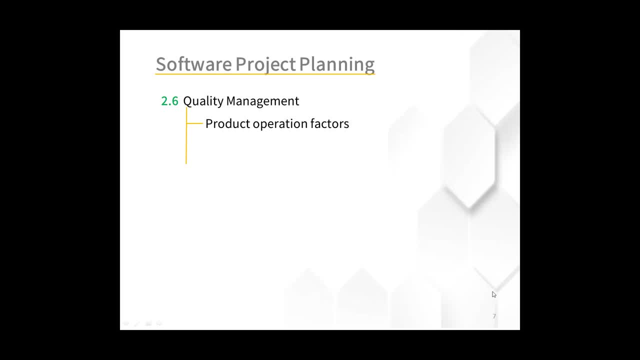 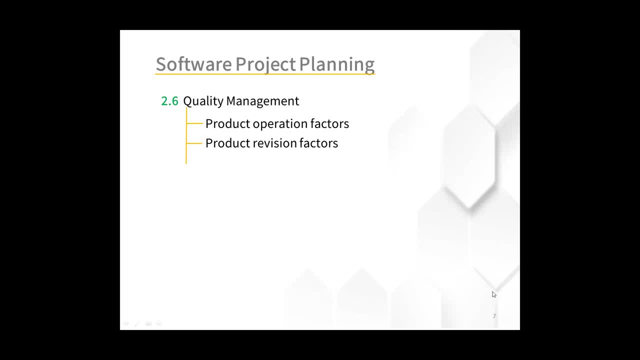 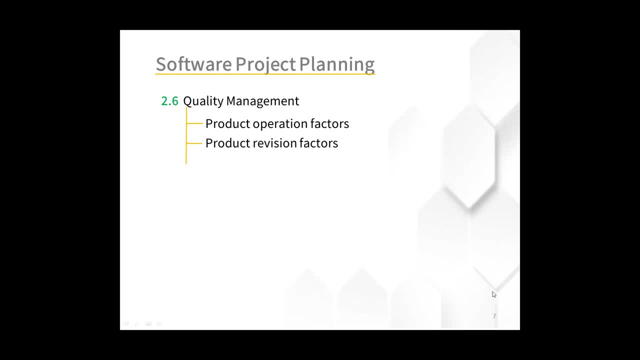 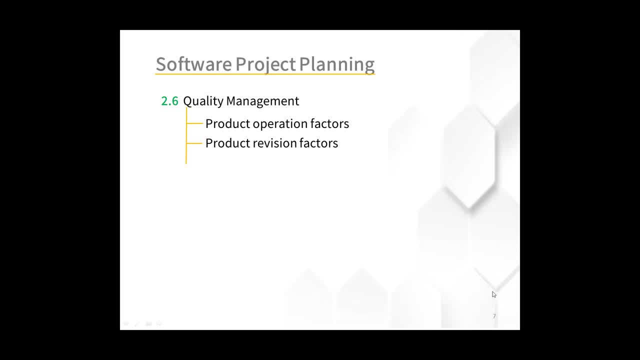 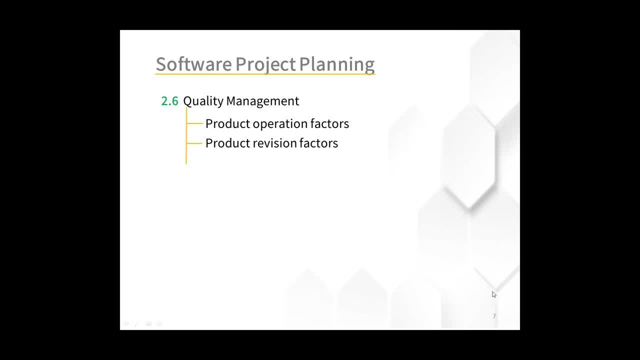 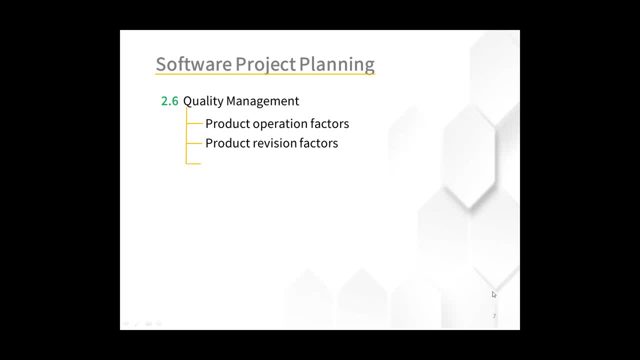 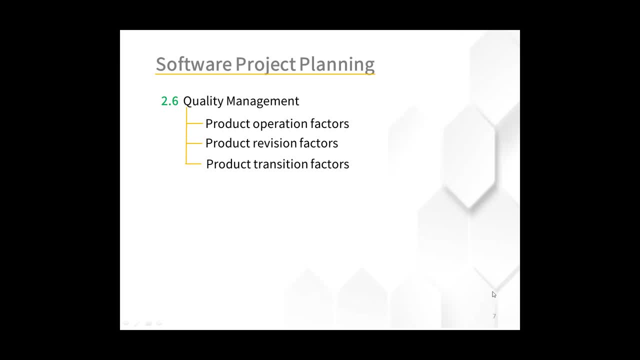 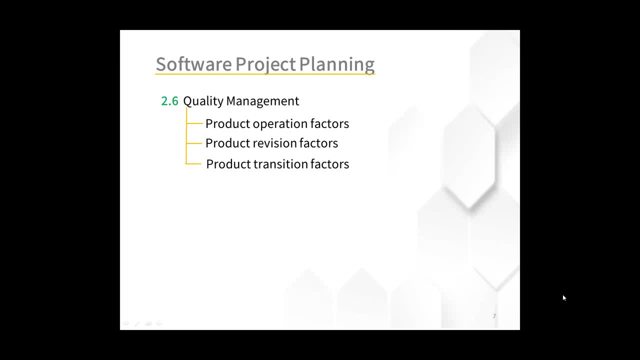 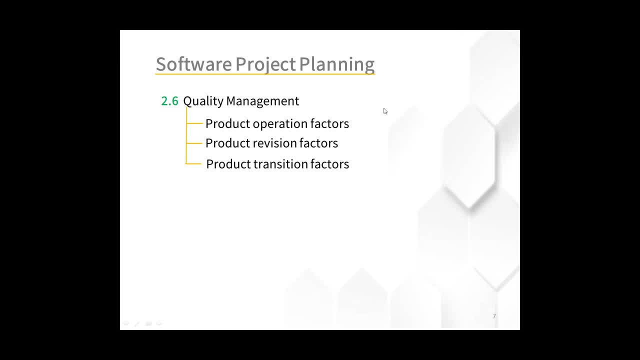 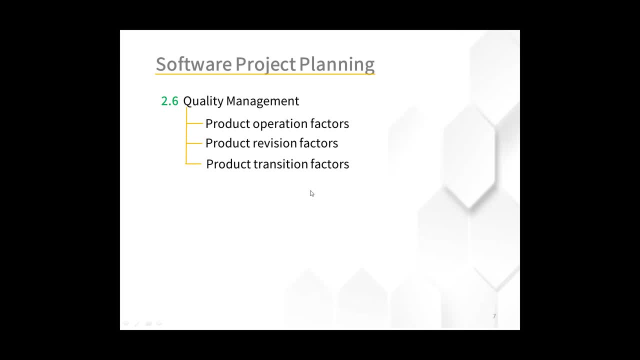 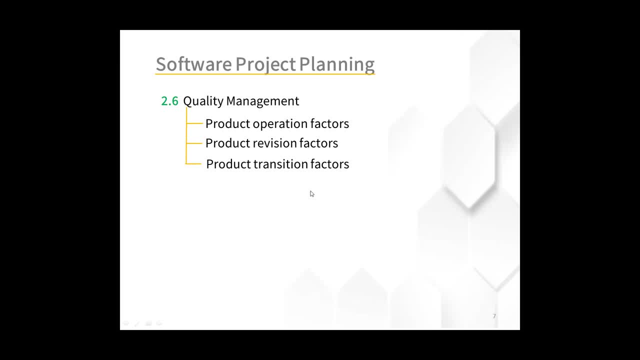 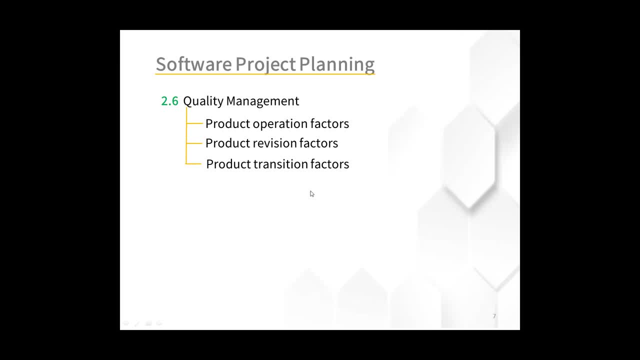 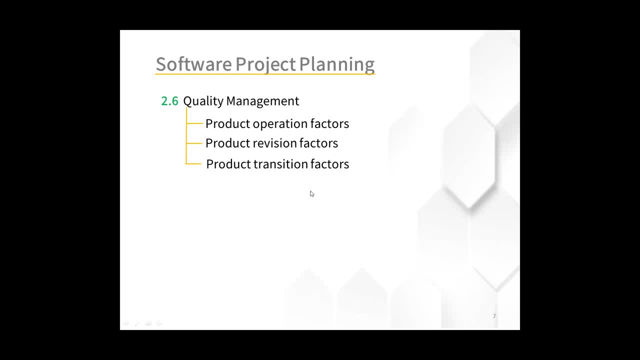 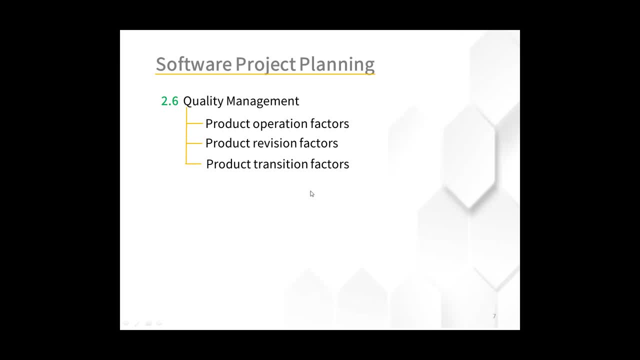 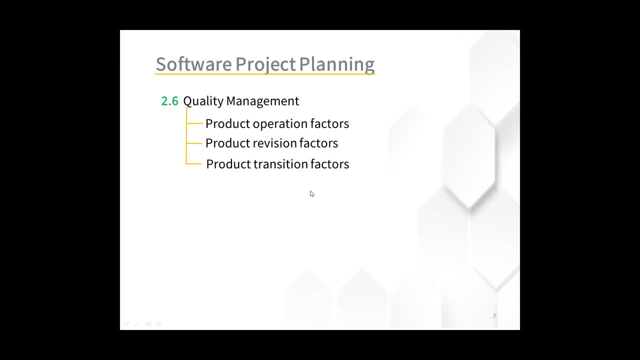 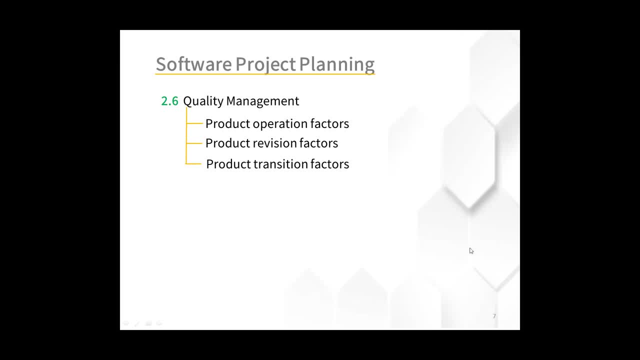 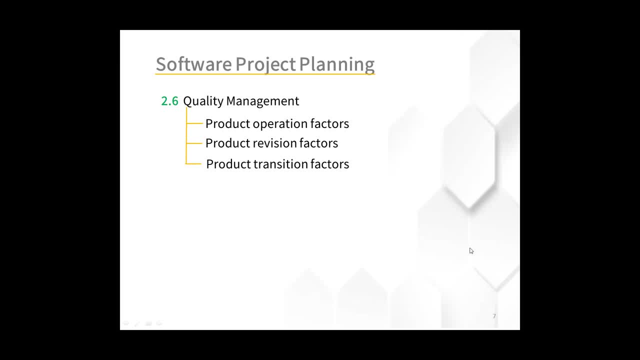 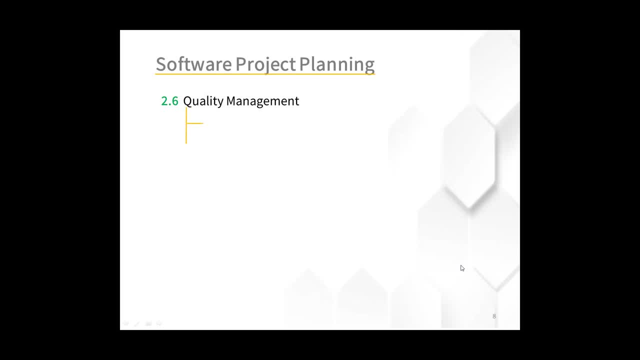 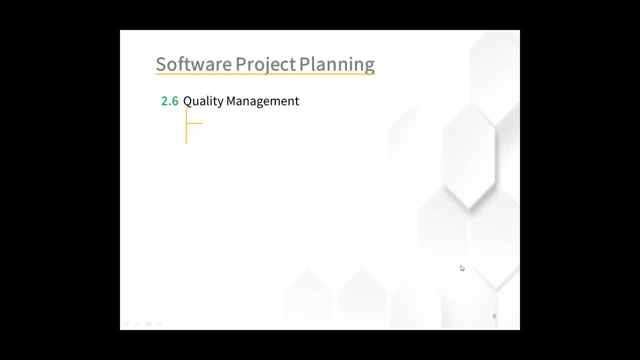 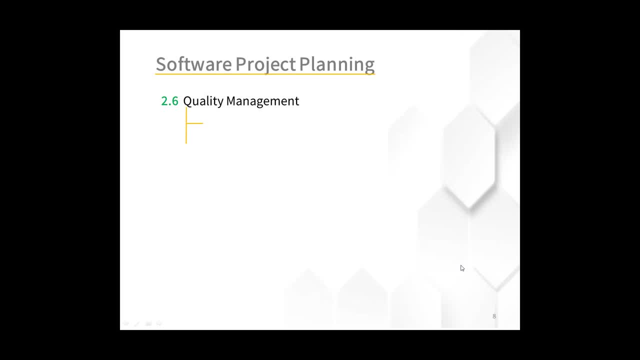 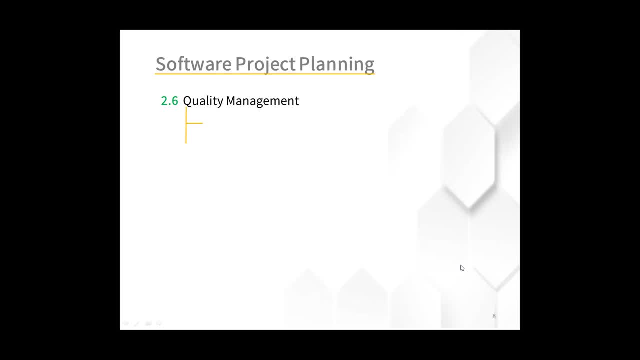 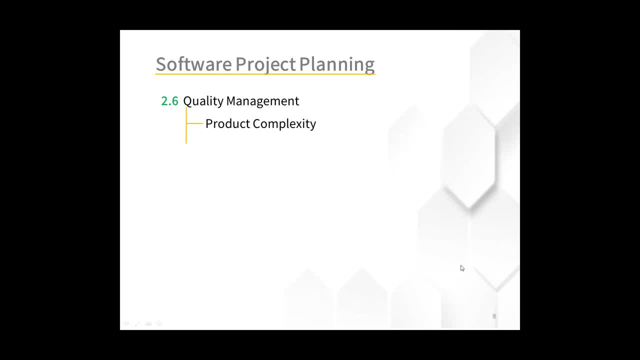 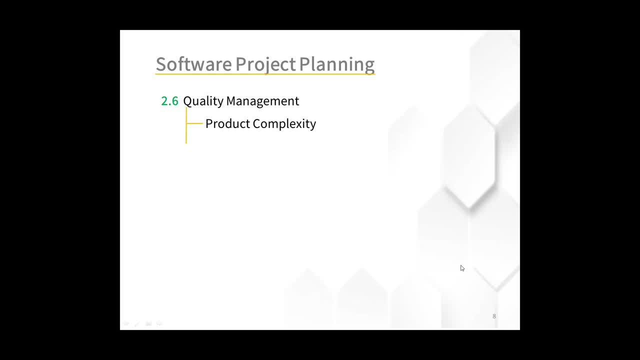 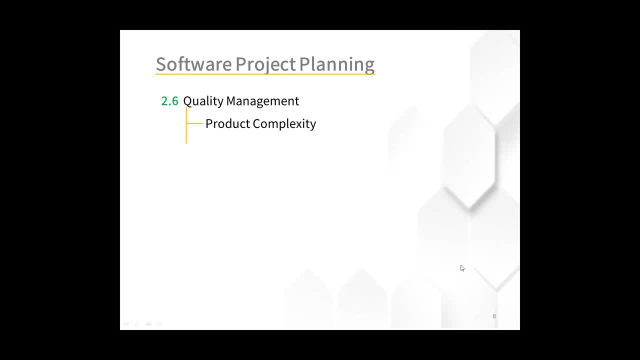 the cost of our product and then we have to determine. We discussed as an example of software product complexity, So our software products are mostly very complex. Software products allows huge number of operational possibilities as compared to other products. For example, take the example of a salt grinding machine or vacuum cleaner or any heavy machinery in any industry, any plant in any industry. 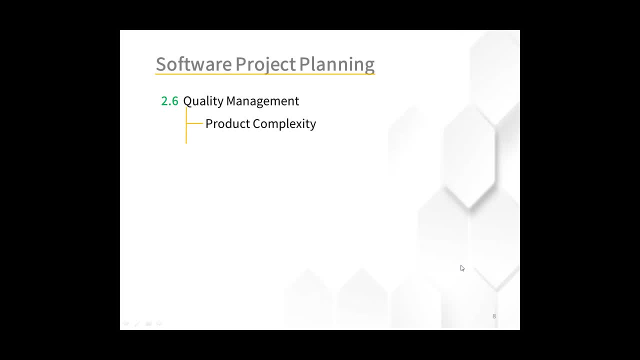 Like the number of operational modes, are very less and manageable as compared to our software product. Our software products allow millions of operational possibilities. So this product complexity is one of the main reason behind the challenging nature And that's why it's very difficult to achieve. 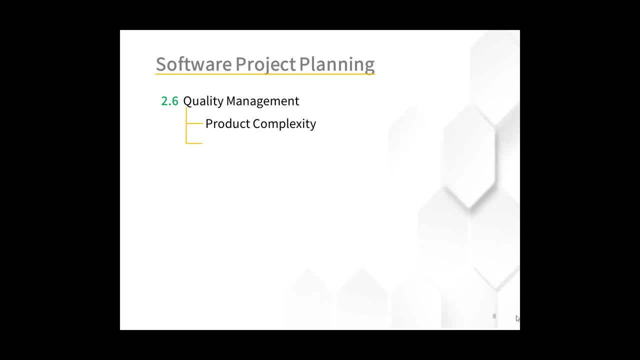 High quality products. Our second reason is product visibility. In industrial products, products are visible, like defects can be detected easily during manufacturing process. Also, missing parts can be easily detected. But this is not the case. This is not the case with software products.